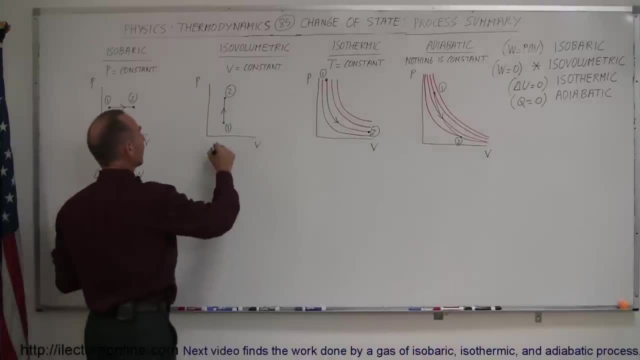 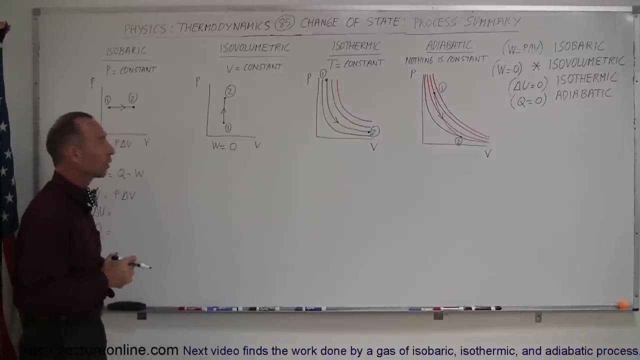 peculiarity there, as you can see, is that the work done is equal to zero because it cannot expand. the gas can only do work if the gas expands. cannot expand cannot do work in an isothermic process, since the temperature doesn't change in the gas, the internal energy cannot change. so here we can. 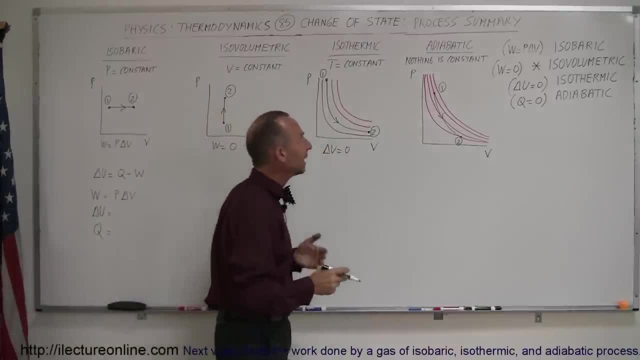 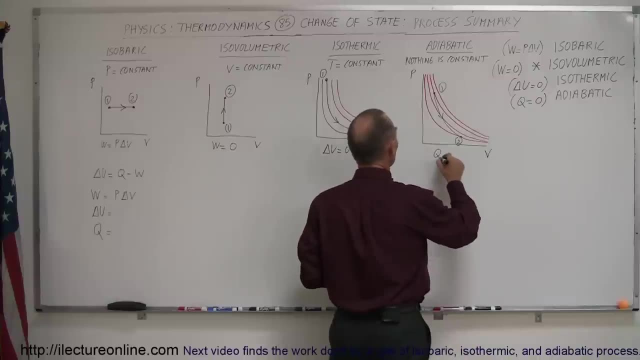 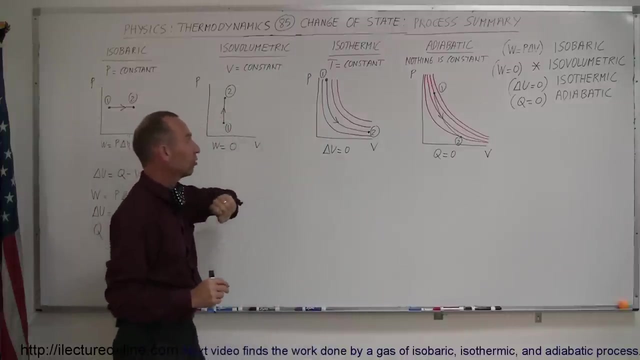 say that delta u is equal to zero. and finally, in an adiabatic process it happens so quickly that q is equal to zero. there's no heat added or removed from the gas, so q is equal to zero. so we have for isovolumetric work is zero. isothermic change in internal energy is zero. 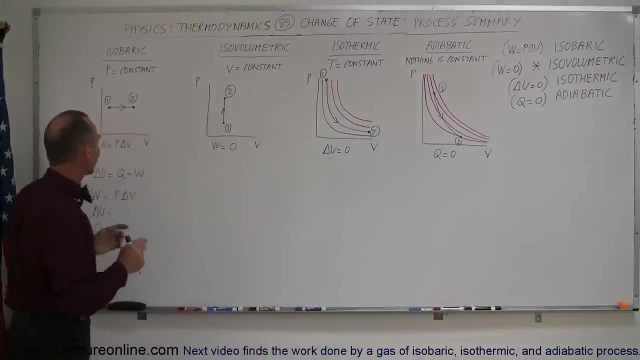 and in adiabatic q is zero, and that, of course, is all related to the first law of thermodynamics, where it says that the change in internal energy of a gas is equal to the heat added to the gas, minus the work done by the gas. 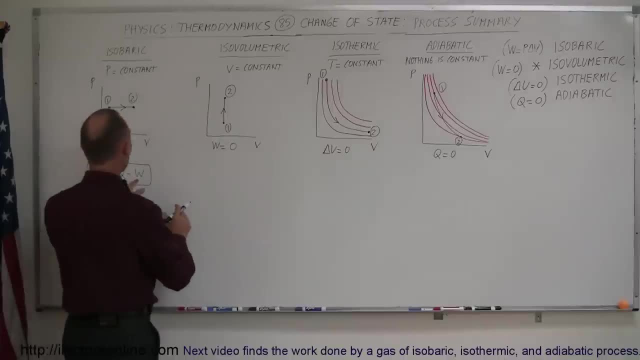 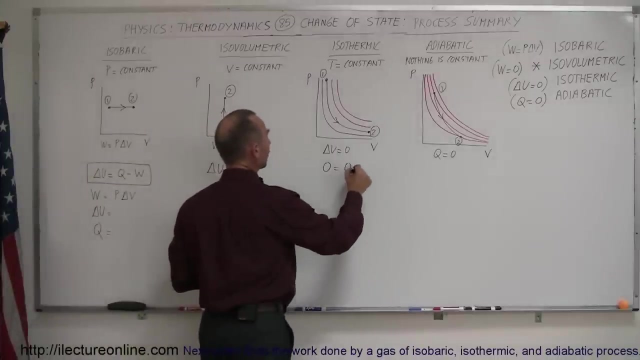 so, in the case of nasa volumetric process, since w is equal to zero, we know that the change in internal energy is simply equal to the heat added to the gas. in the case of an isothermic process, since delta u is zero, then we know that, therefore, that zero is equal to q minus w, so it means that q. 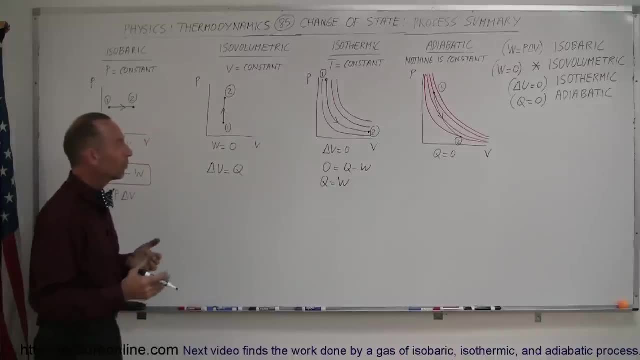 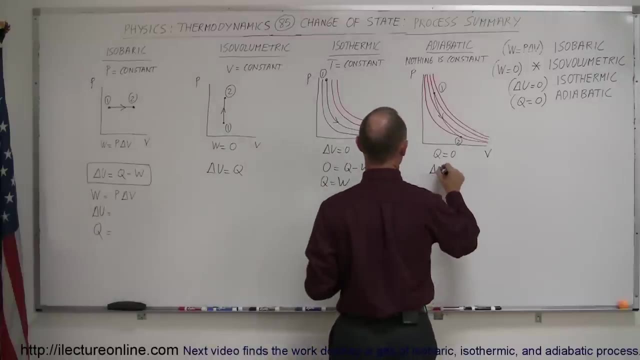 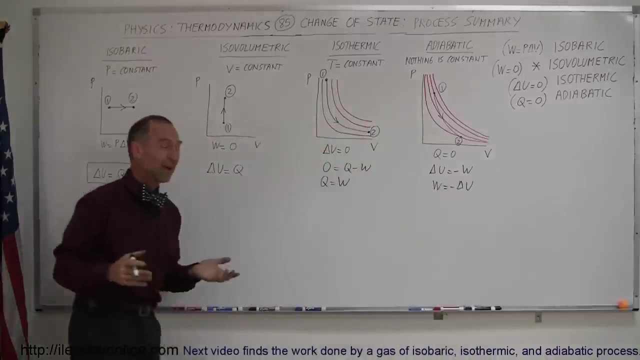 equals w the work done by the gas, equals to the heat received by the gas. and then, finally, here we can say: since q is equal to zero, that means that delta u is equal to minus w, or w is equal to minus delta u, and so, therefore, we can simply find the. 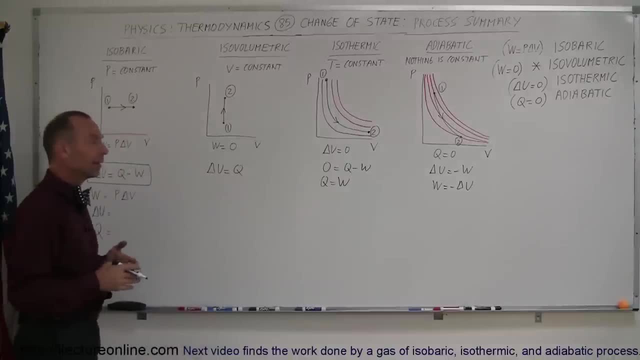 work done by knowing how much internal energy changes. now that's, of course, a little bit more complicated with an adiabatic process, because since none of the three variables are constant, we have to find the relationship between p, v and t in an adiabatic process. okay, how do we define? 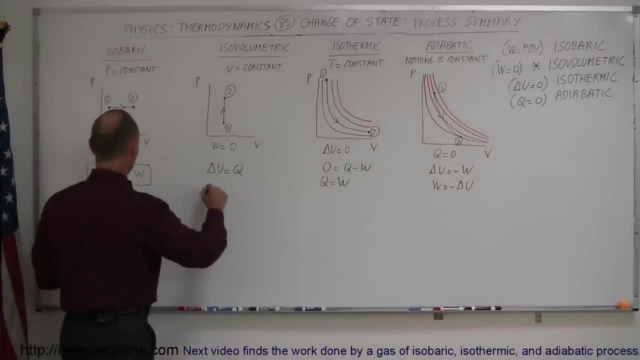 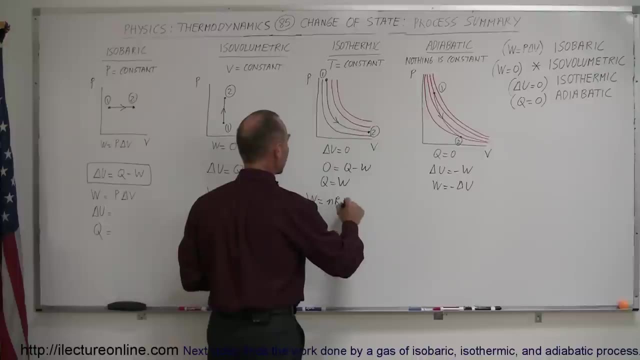 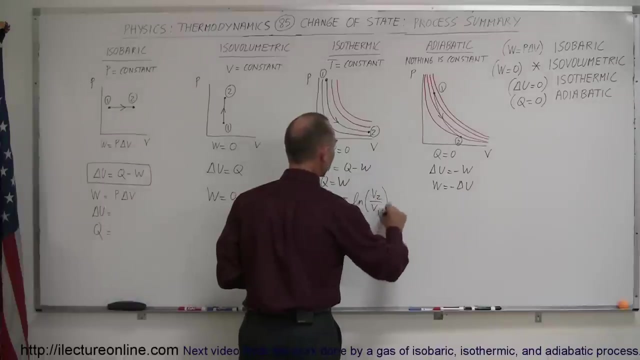 the work done in each case. well, in this case the work done is zero. so that's simple enough: work is zero. in this case, the work done can be defined as n r t, because t doesn't change. that's a constant number times the natural log of the ratio of the volume that you end up with divided by the volume you started with. and if 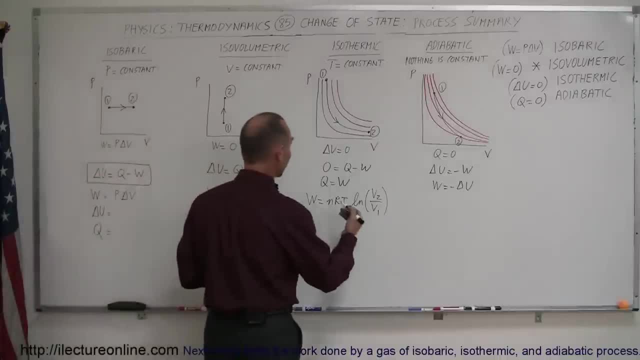 those if temperature is not known. in this case you can also replace that by p1 times v1, so work done can also be expressed as p1- v1. so that's the ratio of the volume that you end up with times the natural log of v2 over v1. or you can say that work done is equal to p2 v2 times the. 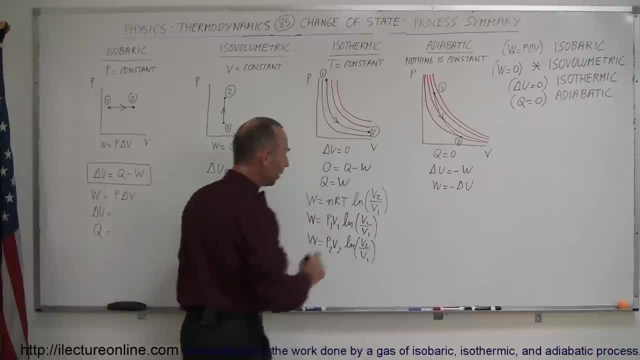 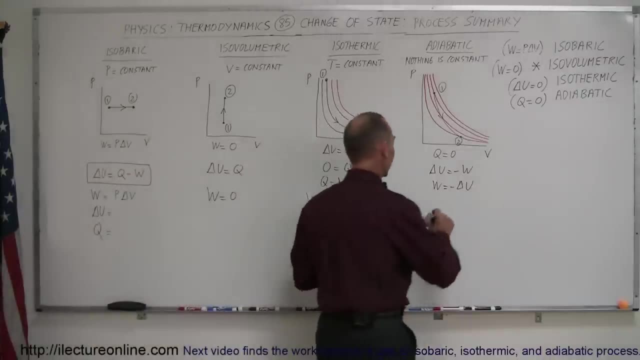 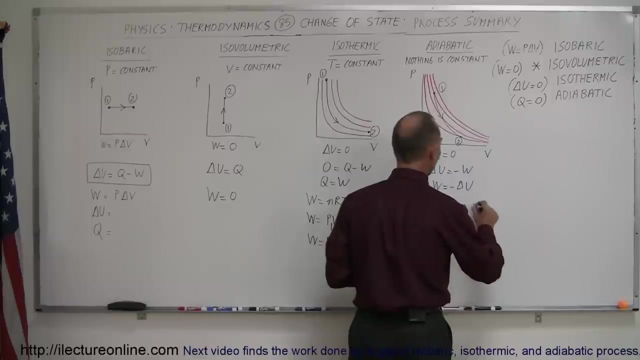 natural log of v2 over v1. so there's a lot of different ways to figure out the work done in an isothermic process. the work done in an adiabatic process can be defined as the negative of the change in internal energy, which can be defined as the number of moles times c, sub v, times the change. 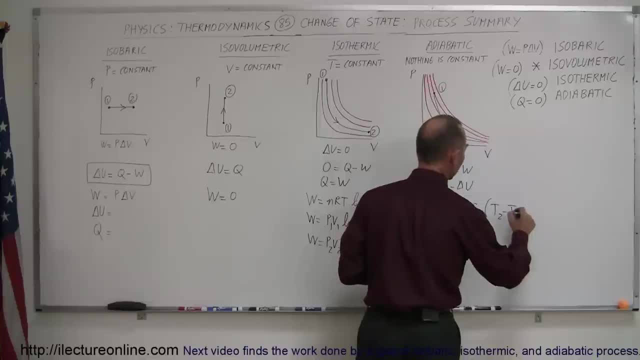 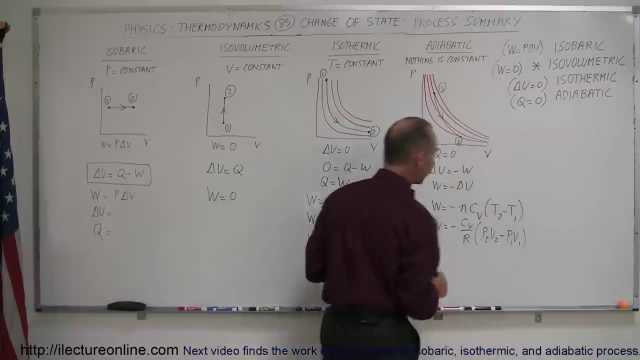 in temperature, which is t1 minus t2 minus t1, and, of course, if those are not known, you could also express the work done as being equal to minus c sub v over r times p2 v2 minus p1 v1. so you can find the work done. 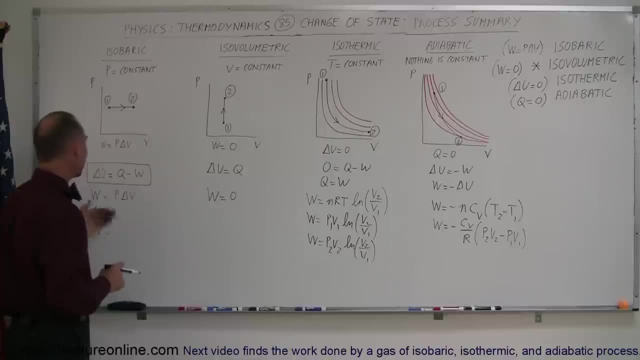 in either way, with an adiabatic process, the change in internal energy is always going to be the same for every uh. every uh i should call thermodynamic process. i'm kind of stumbling over my words here, but in general the equation always going to be n, c, sub v times, delta t. so here, since pressure is constant, that 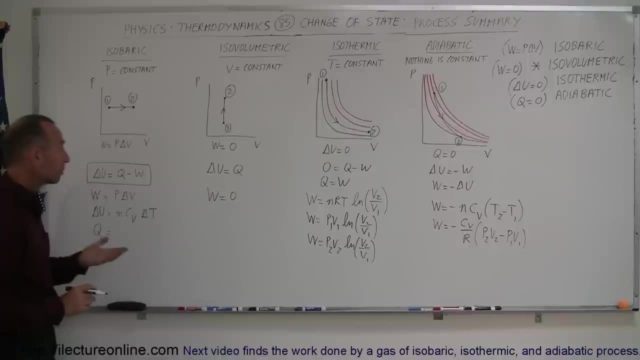 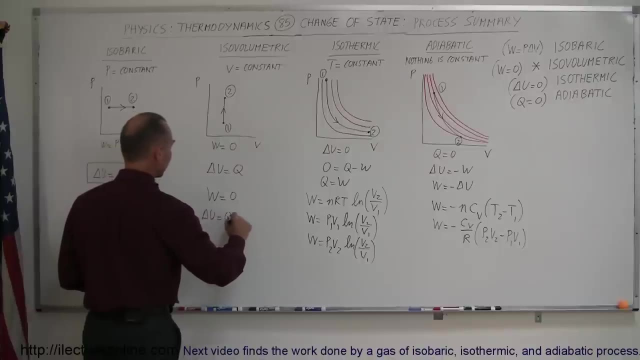 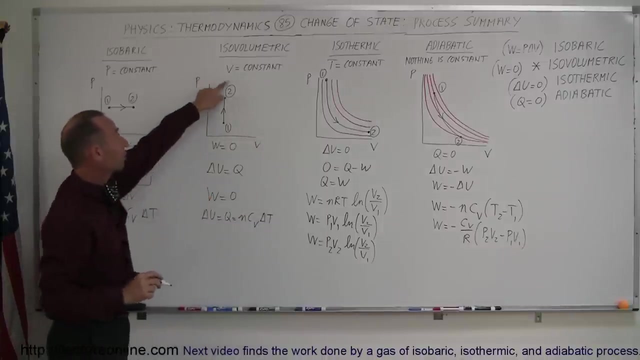 is pretty well the only way you can do that. in the case of an isovolumetric process, delta u is equal to q, and so we can also say that delta u here, which is equal to q, which is equal to n, c, sub v, delta t, and notice that in the case, in the case of a isovolumetric process, where v is constant, 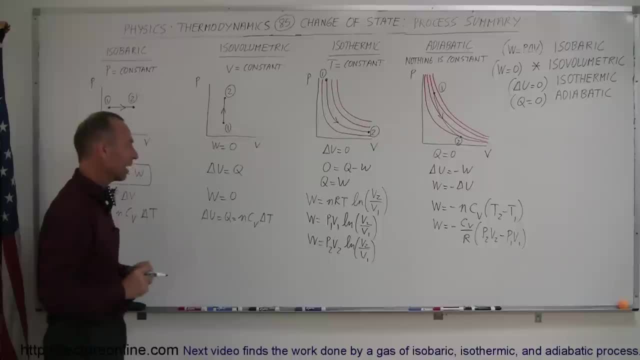 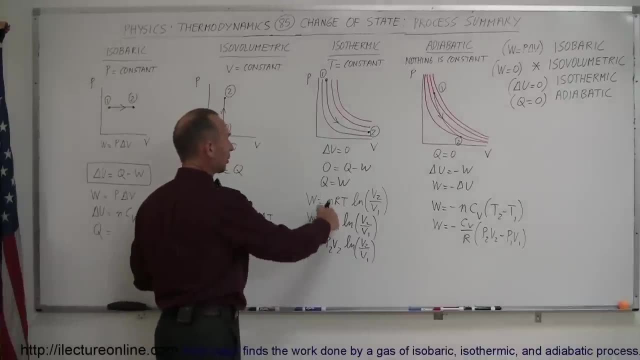 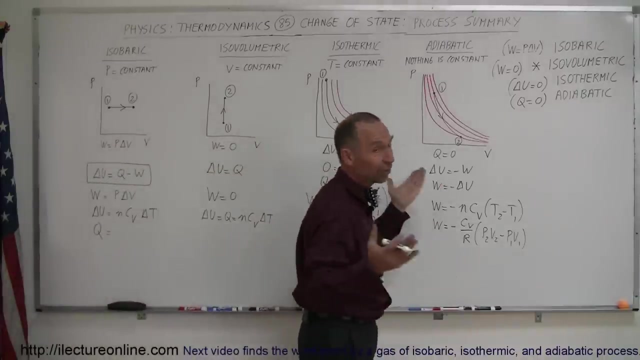 q is also n c, sub v, delta t, which is not always the case in an isothermic process. uh, delta u is zero, so q is simply equal to the work done. so whatever you find out is the equation for work. that's also the equation for q, and then here q is always equals to. 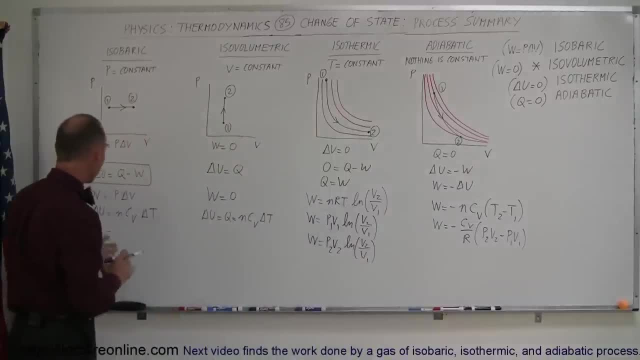 zero. so there we don't have to worry about the heat added to a gas. finally, q here in an isobaric process is a little bit different than there. here it is n, c sub p, delta t, and notice that c sub p. So the heat added to a gas is different if it's an isobaric process compared to when it is an isovolumetric process. 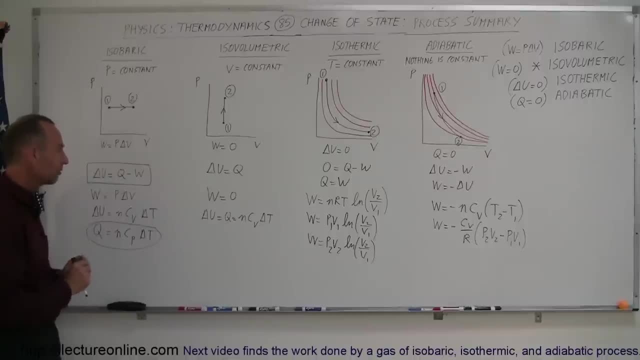 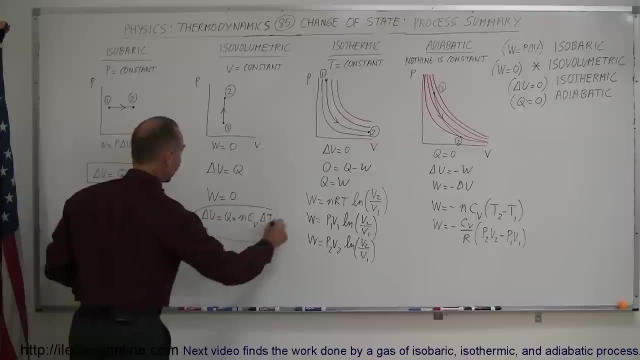 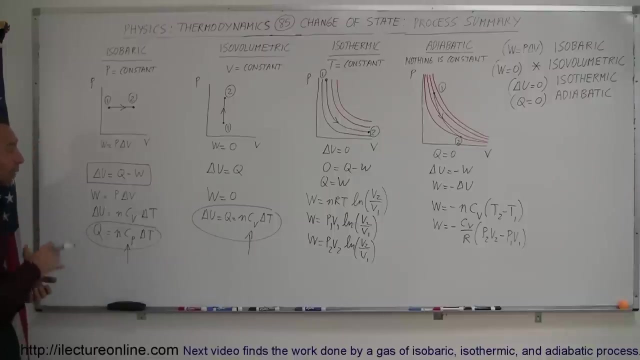 And don't forget that, because sometimes you'll have to figure out Q in either an isobaric or an isovolumetric process, and it is indeed different, So be careful that those are not the same. It does depend. The heat added to a gas does depend upon how the gas expands or whether or not the gas expands at all.